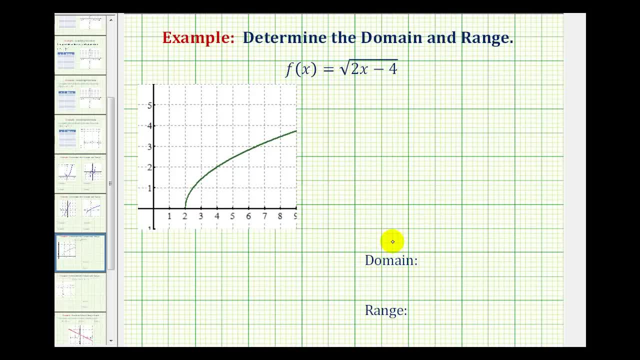 like this and remember: the domain is a set of all possible x values which occur on the horizontal axis and the range is a set of all possible y values, and y values occur along the vertical axis. So to graphically determine the domain, we want to project the function onto the x axis. 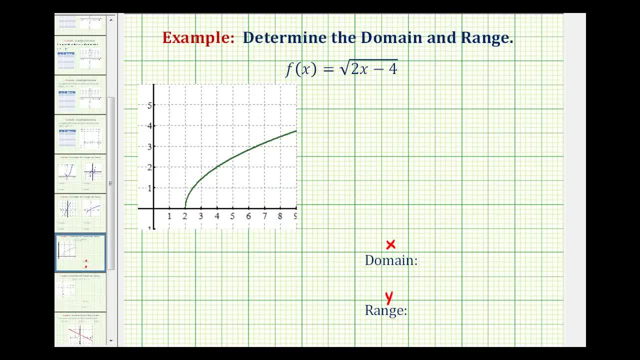 or determine how the function behaves horizontally. What I mean by that is to determine the domain. notice how the leftmost point of the function would be this point here, When x is equal to positive two, and then from here all the x values move to the right or increase. 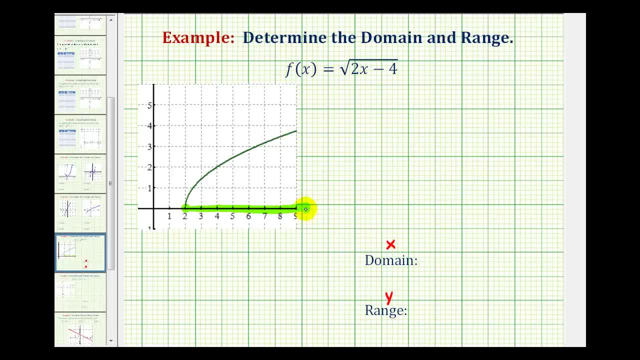 So the domain would be from positive two approaching positive infinity, And we can express this two ways. We could say that x is greater than or equal to two, or using interval notation, we could say the interval from two to infinity, where it's closed on two or it includes two. 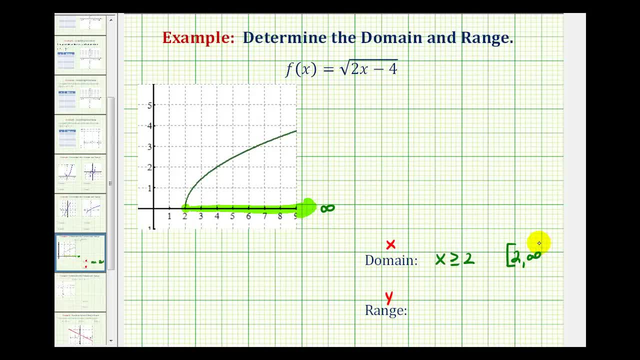 So we have a bracket here And then a rounded parenthesis for infinity And then for the range. we want to project the graph onto the y axis or determine how the function behaves vertically. Notice how the lowest point on this graph would be right here when y is equal to zero. 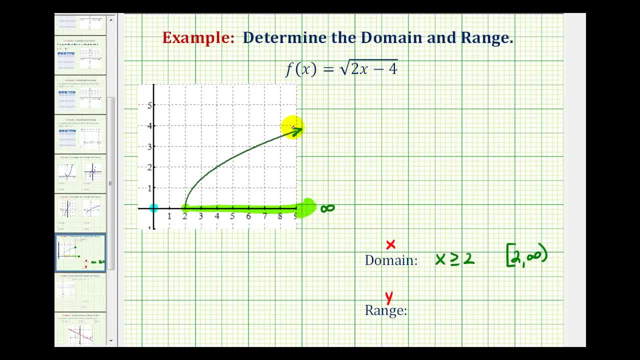 And then from here, even though the graph is moving quite quickly to the right, it also continues to move upward. So the range would be from zero approaching positive infinity Along the y axis. So the range would be: y is greater than or equal to zero. 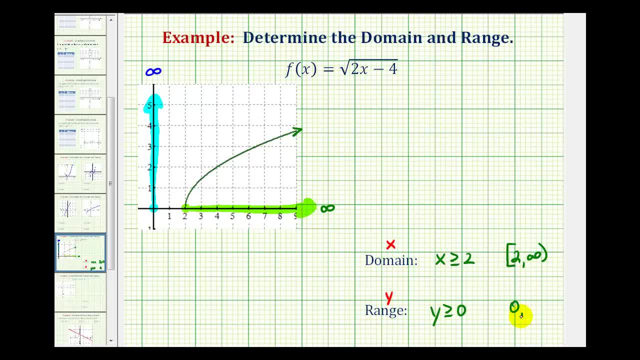 Or using interval notation we could say the interval from zero to infinity, where it's closed on zero and we have a parenthesis on infinity. But of course it does take some time to graph the function. So we can use what we know about a square root to determine the domain in the range without a graph. 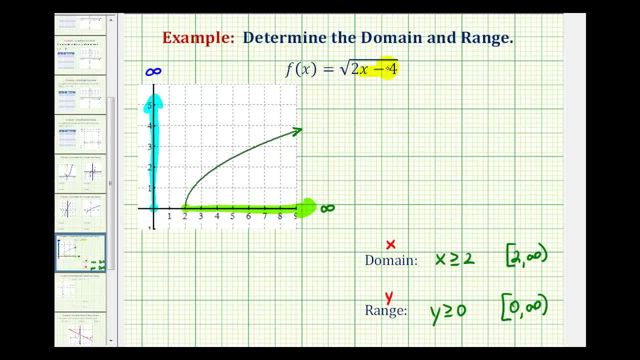 Let's see if we can do that. We know that to evaluate a square root, the radicand, or the number underneath the square root, must be greater than or equal to zero. It can't be negative, because that would produce an imaginary number. 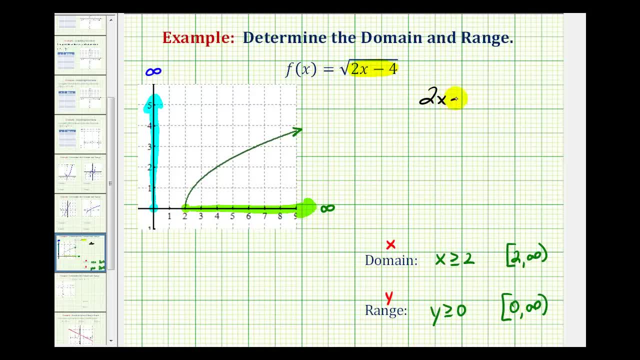 So if we recognize that 2x minus 4 must be greater than or equal to zero, we could solve this inequality and find the domain this way as well. So if we add 4 to both sides, we would have 2x is greater than or equal to positive 4..